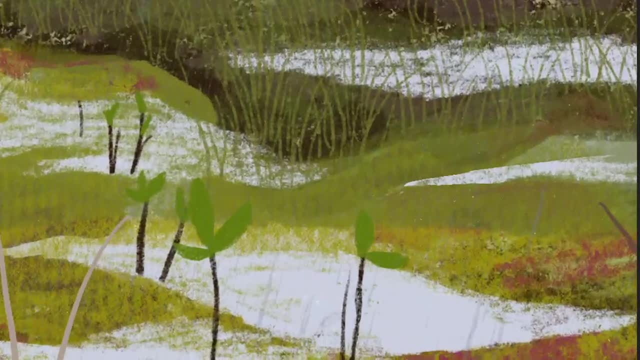 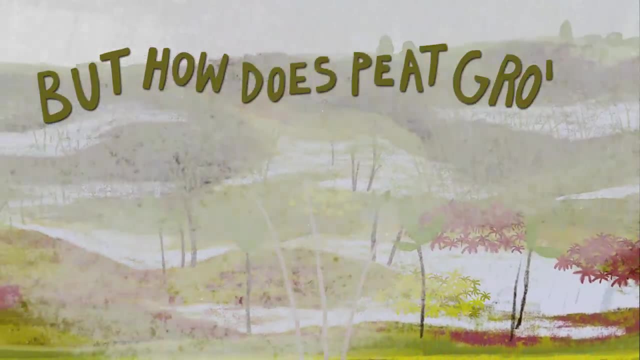 perfect for the rainy Irish climate. The vegetation that forms the peat is dominated by a special type of moss called sphagnum, which thrives in water. But how does peat grow and why are the peatlands so deep? The difference with sphagnum compared to other plants is that 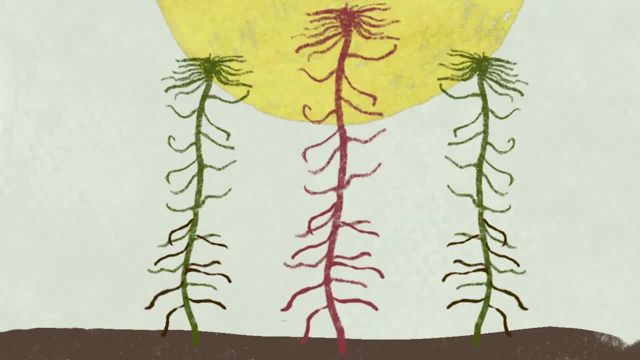 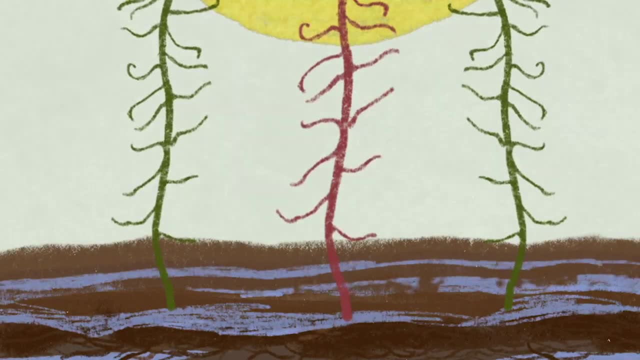 it has no roots. The sphagnum grows up towards the sun and as it does this, the stem becomes part of the bog. This results in layers of organic vegetation forming on top of each other, creating a peatland. Carbon is trapped between these layers like a sponge. 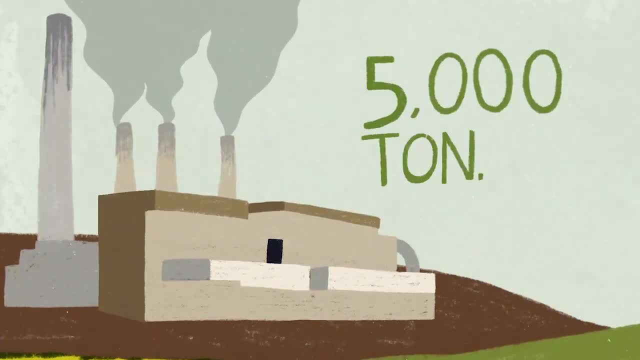 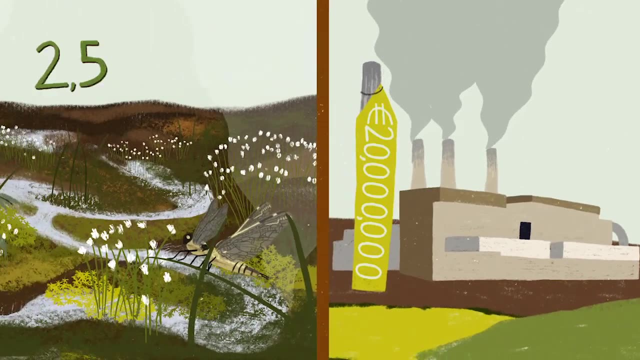 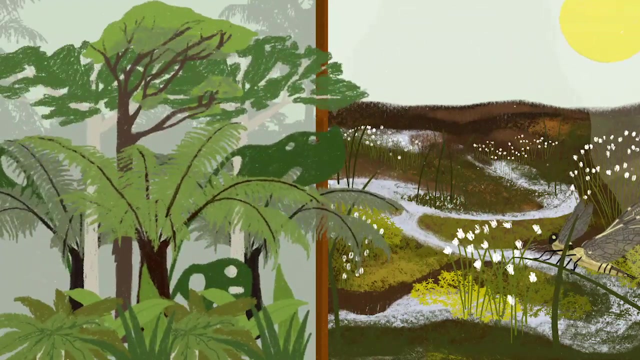 To build a carbon capture station taking in 5,000 tonnes of carbon each year would cost around 20 million euro, Or you can let 2,500 hectares of natural bog do the work for you for free. This special moss has stored an enormous amount of sunlight in its peak soil over the years. 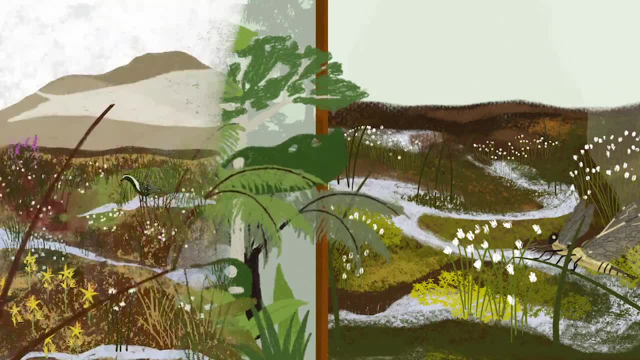 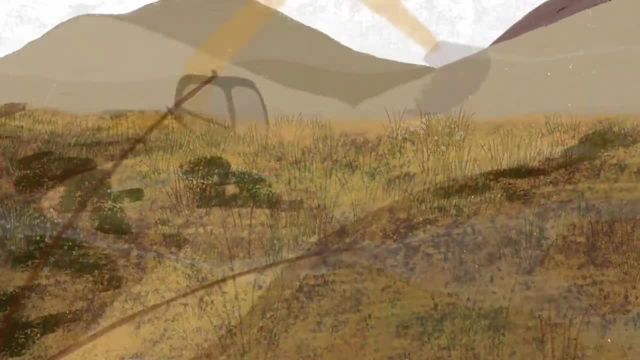 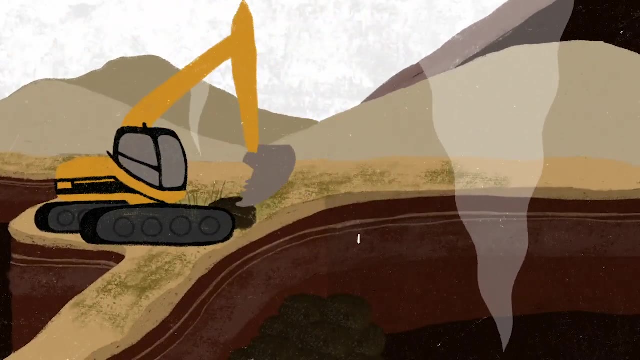 much more than a tropical rainforest, for example. Sphagnum and the wet environment it grows in are huge assets in our fight against climate change. However, burning or draining peatlands can be dangerous. Sphagnum peatlands destroys this delicate, damp ecosystem and releases carbon back into our 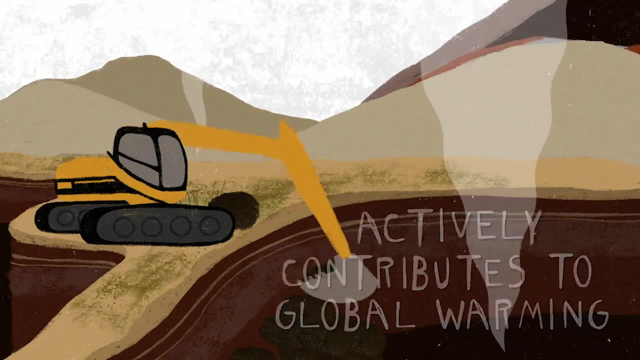 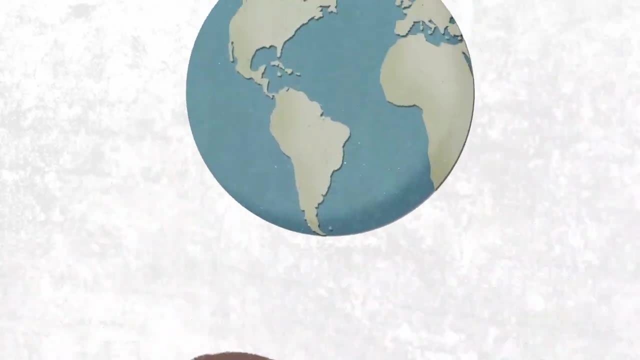 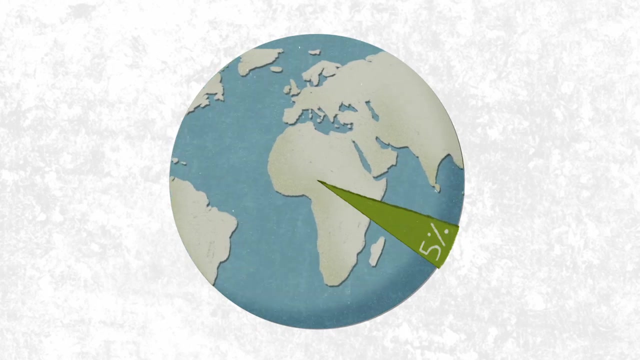 atmosphere. This actively contributes to global warming. A hectare of drained peat emits around six tonnes of CO2 per year, equal to the emissions of one and a half cars. Globally, as much as five percent of the annual greenhouse gas emissions come from damaged peatlands. despite the fact, peatlands 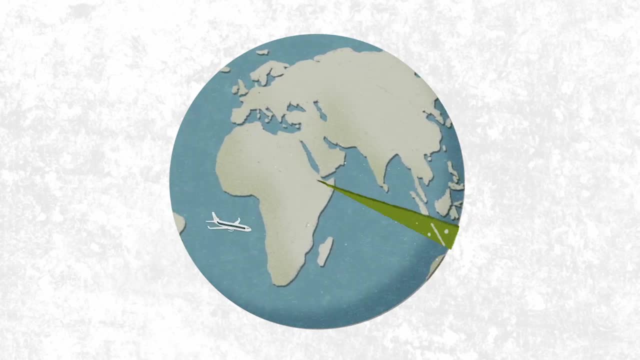 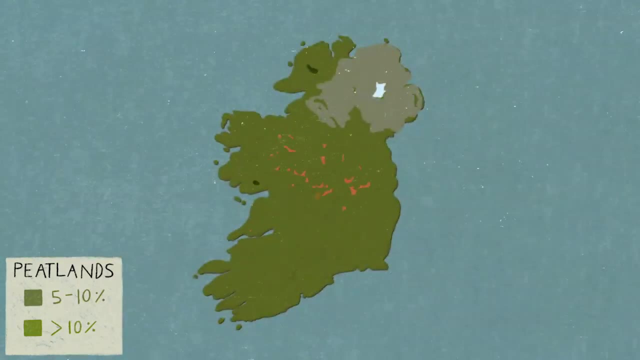 cover only three percent of the earth's land surface. This is what we call a carbon capture station. This is more than the emissions from aviation. This is an issue of international concern, and countries with large peatland cover, like Ireland, have a special responsibility to conserve these invaluable ecosystems. 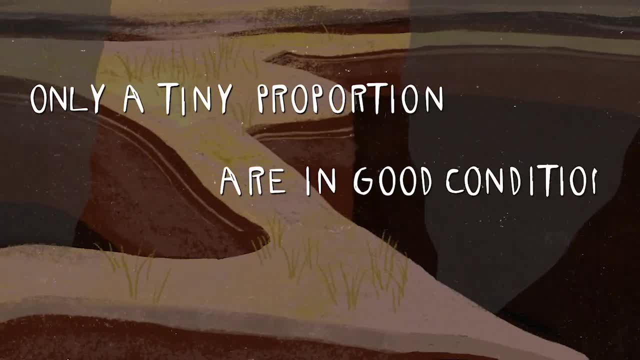 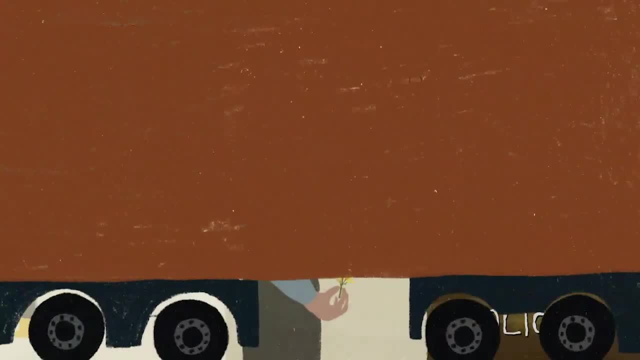 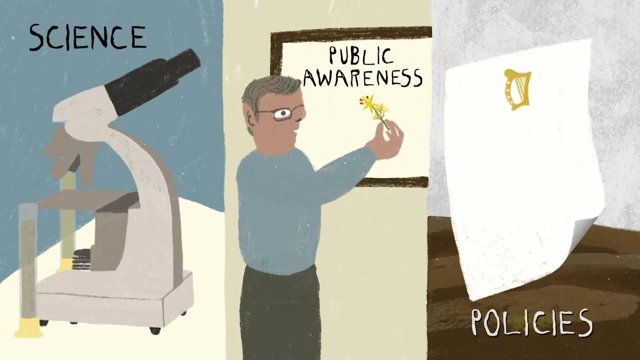 Only a tiny proportion of these bogs are in good condition and annual emissions from deteriorating Irish peatlands are nearly as high as those from transport. But with advances in science, public awareness and government policies, we are restoring peatlands back to their natural boggy state.